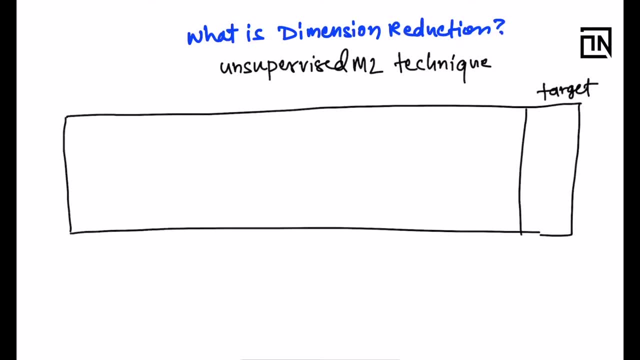 you have one target variable and there are multiple predictors: Predictor 1, predictor 2, predictor 3, so on and so forth till predictor 500. So there are 500 columns in your data and one target variable. But hold on, you just said that it is an unsupervised machine learning. 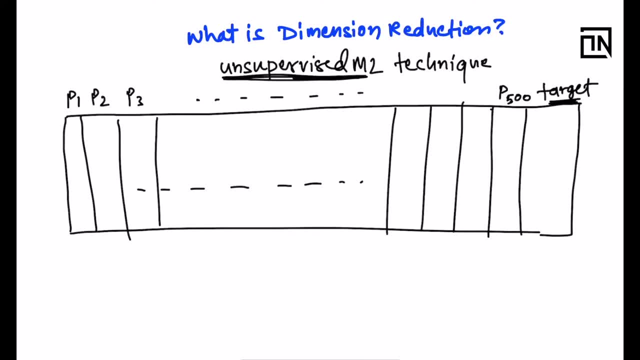 technique. So how come this target variable is coming into picture? So this target variable doesn't come into picture when you do dimension reduction. So over here, the problem which you will face in using this data to fit your machine learning models is you need to take into account all the 500 columns, Okay, and when you take 500 columns, 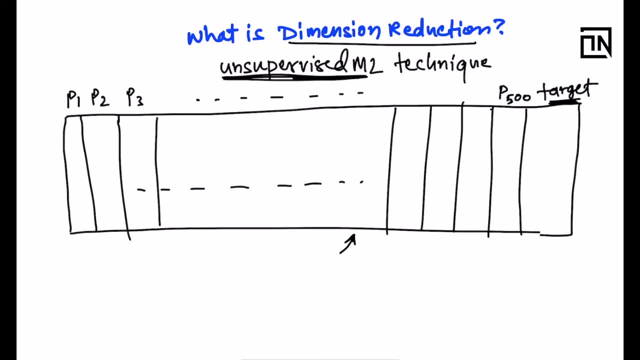 into account this kind of data or more. let's say you have 1000 columns or 2000 columns. these kind of scenarios are very common in text mining. So whenever you are doing natural language processing, you're trying to create. 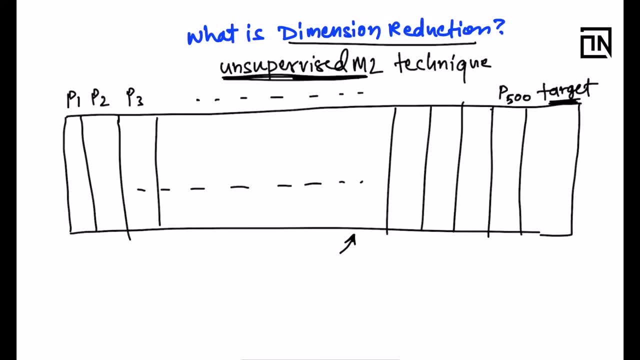 a model, let's say for ticket classification. so the ticket description data needs to be converted into numeric form and then each word will represent one column, also known as the document term matrix. in such kind of data sets, thousand columns or two thousand columns of predictors is very common. 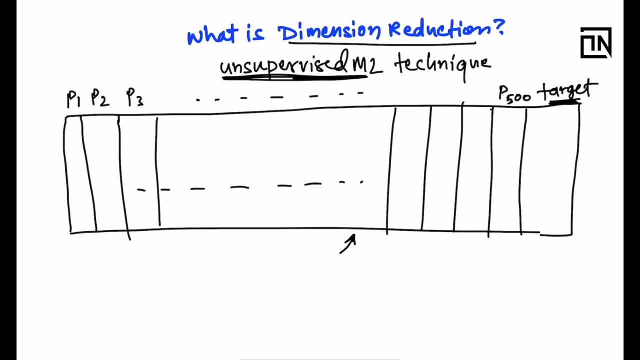 so in such scenarios, let's say, if you use that data to try to fit through a machine learning algorithm, it will take large amount of time and it will be painfully slow. so what you can do is, instead of fitting these 500 columns all together, is there a way in which you can shrink these 500? 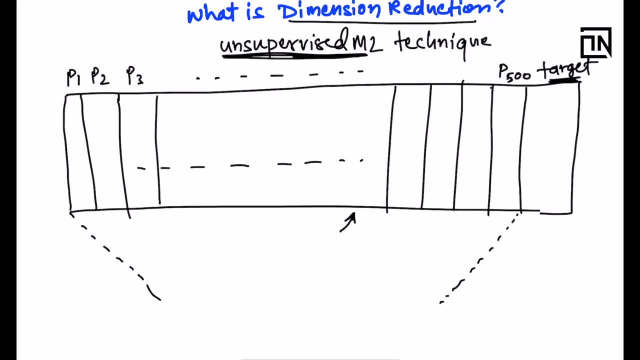 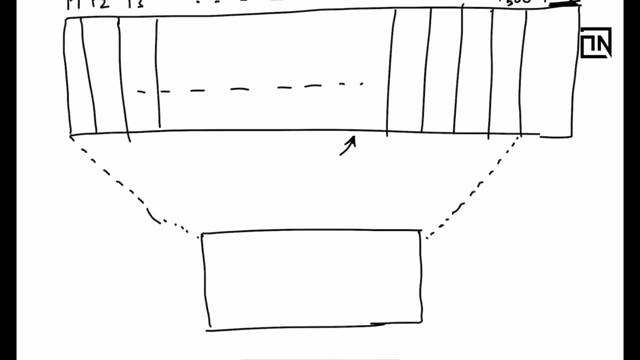 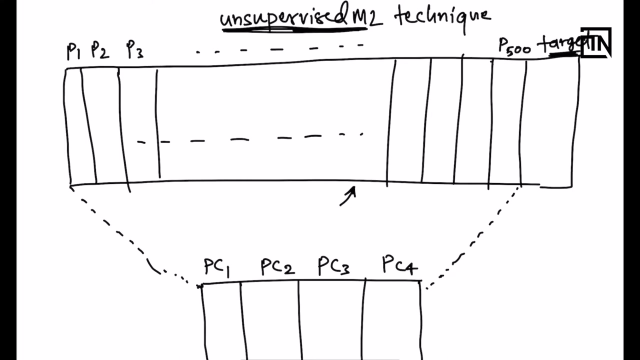 columns, which you have 500 predictors. i am shrinking the number of predictors only with some smaller number of columns. let's say, let me call these columns the very famous principal components. let's say principal component one, principal component two, principal component three and principal component four. so i am representing these columns, these 500 columns, with just four columns, or maybe thousand. 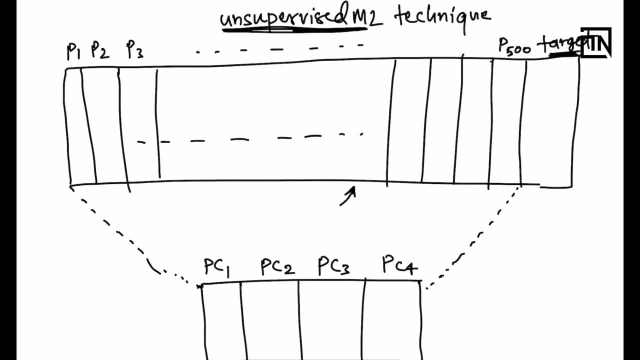 columns with four columns or five columns or ten columns? how do we decide these columns? it is based on the algorithm to algorithm. okay, so we will discuss that going further, but this is the overall idea. i am doing some work only on the predictors data, so i am shrinking the predictors representing large number of predictors with smaller number. 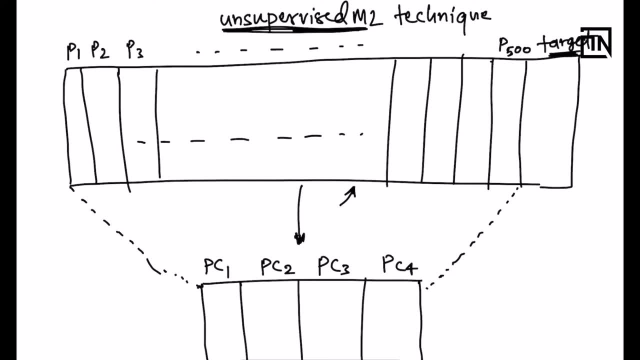 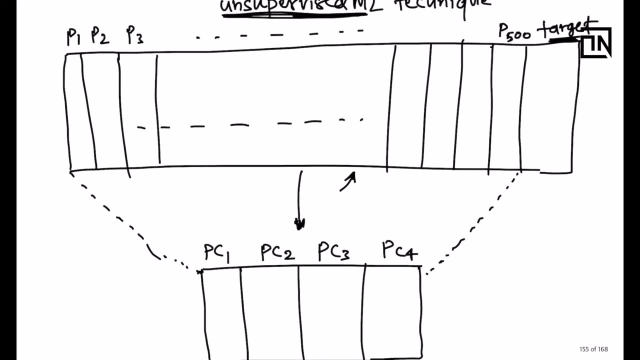 of predictors. how many predictors should i choose to represent these 500 predictors? this is also something which varies from algorithm to algorithm, which we'll discuss further. okay, so once i have given this representation of 500 columns, with just 400 columns, now i can bring in the target. 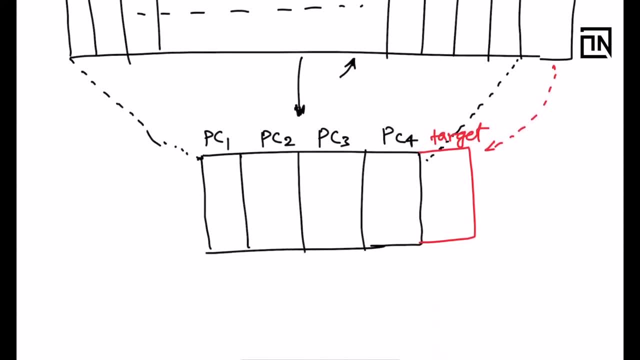 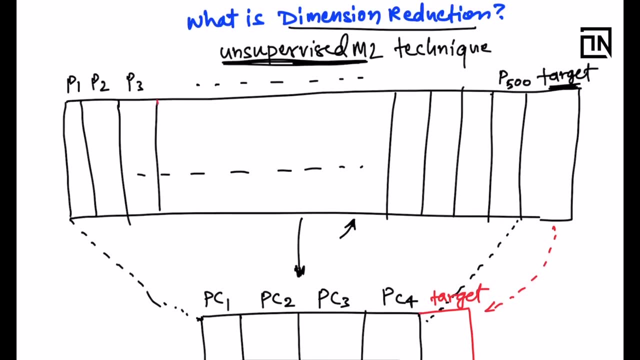 variable create this new data. so now this new data is a representation of the overall data which was having high number of dimensions. dimension means what columns? so these are nothing but dimensions. every column represent one dimensions. so if there are so many dimensions in my data because of xyz reasons, i can somehow represent it with smaller number of dimensions. 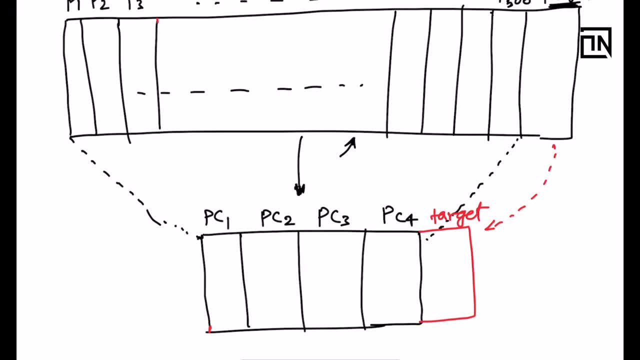 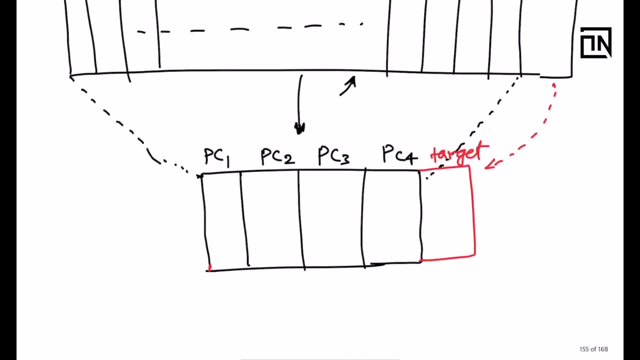 or smaller number of columns, and these dimensions could sometimes be called as factors and sometimes called as principal components, etc. so different algorithms will name it differently the way they combine it. okay, so once you do this now, you have a new data and on this data you can fit your machine learning algorithms. 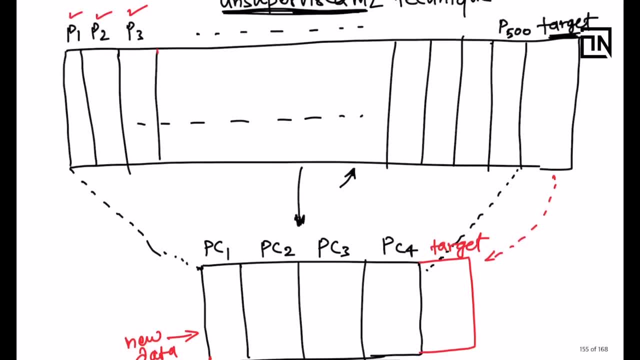 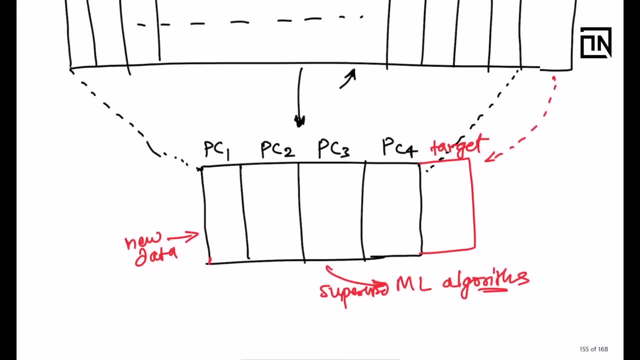 supervised machine learning algorithm because, let's say, the target variable is there, then definitely, either you are doing regression or you are doing classification. so what we are going to do is we are going to do the same thing. we are going to do the same thing. so, whatever is the scenario, if you are trying to predict something which is in the number, 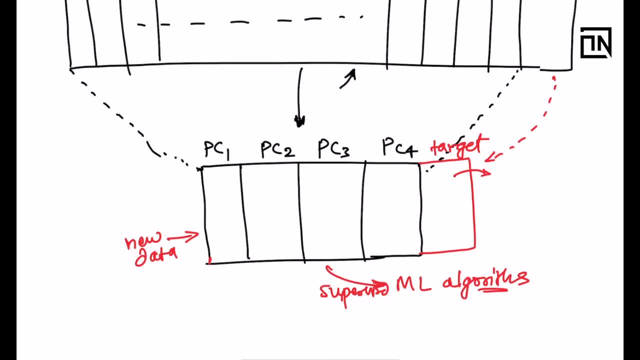 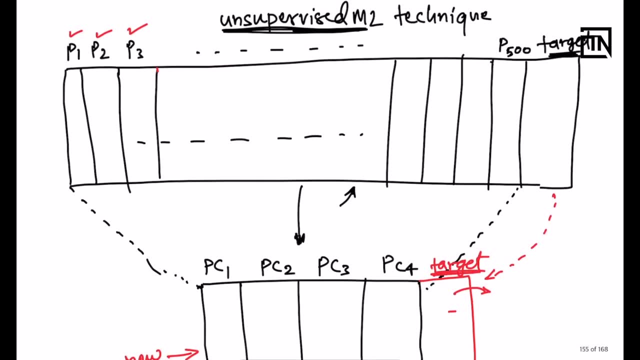 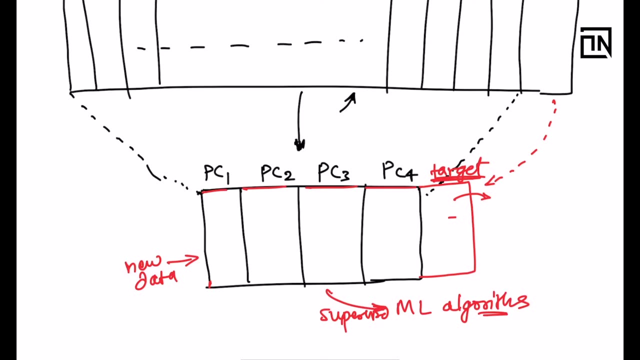 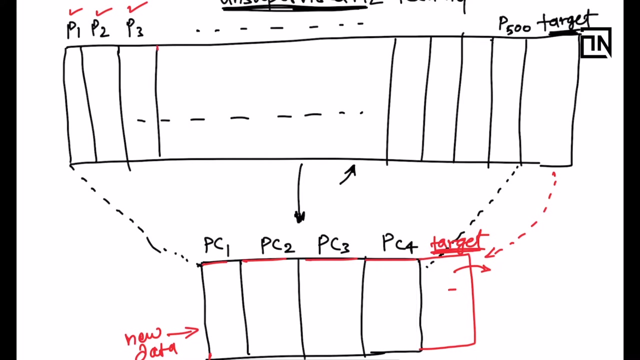 then you will fit: supervised regression machine learning or, if it is a class, then supervised classification machine learning, depending on the target variable. okay, but the crux is, your predictors are now shrinked to a smaller set of columns. okay, the whole journey of how these predictors are shrinked to smaller set of columns. this is something what we call as 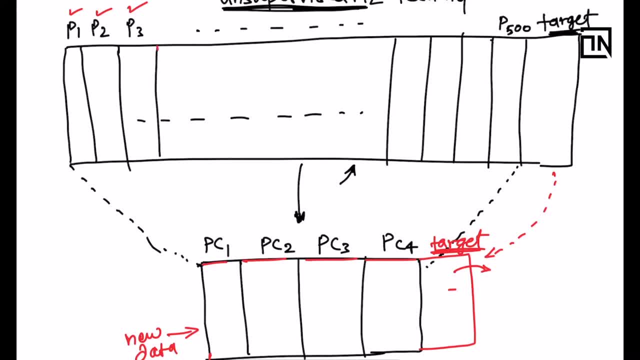 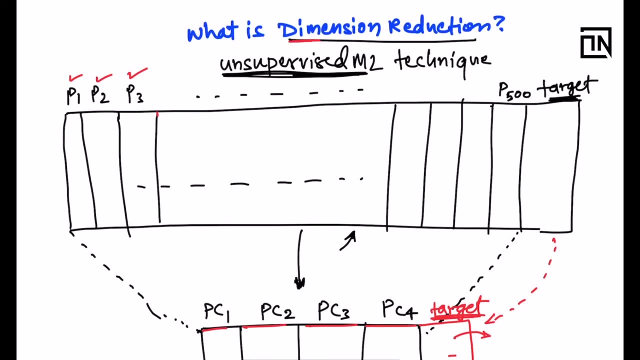 different. this is something which is very different for different algorithm. for example, in factor analysis, it will happen differently. in principal component analysis, it will happen differently. or independent component analysis, it will happen differently, so on and so forth. so what is the need for dimension reduction? why do we require this activity to be performed? 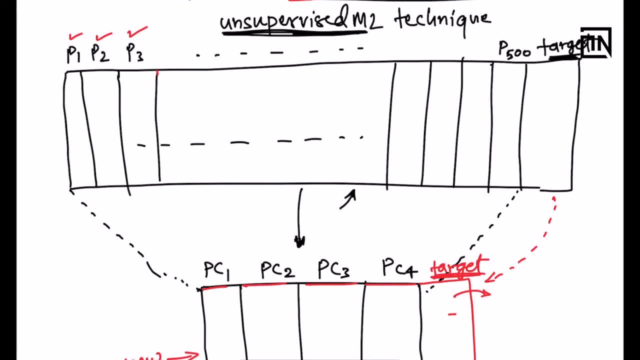 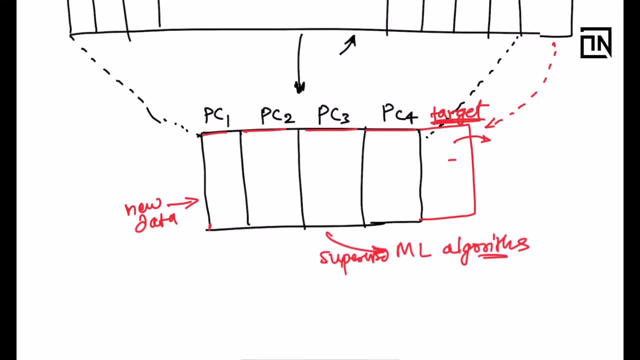 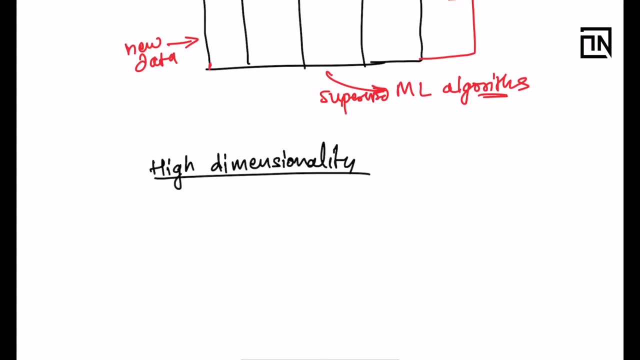 because if you choose all the predictors, then your model training on this old data or the raw data, the model training will be very slow. so if your data has high number of dimensions, high dimensionality, what we call if your data is suffering from high dimensional, high dimensionality, 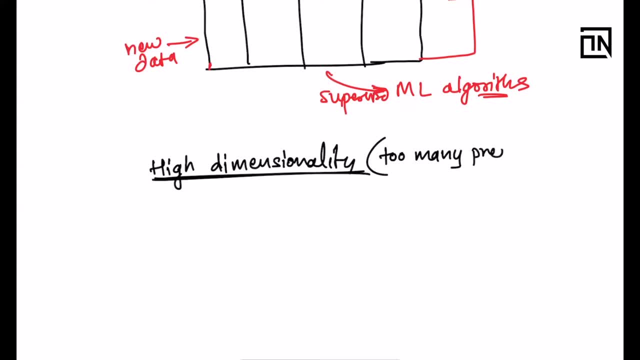 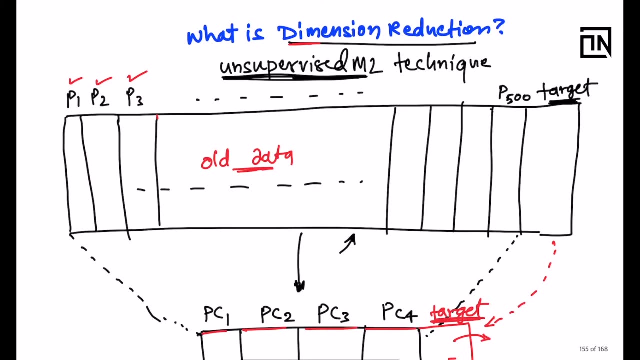 or too many, call too many predictors, because target variable is always one. so, if this is the issue, what it will impact on your machine learning training is, first of all, it will be slow- and this is no brainer- if you have more columns. in order to learn more, you need. 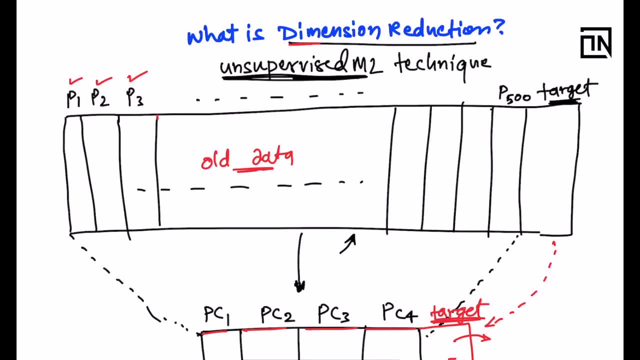 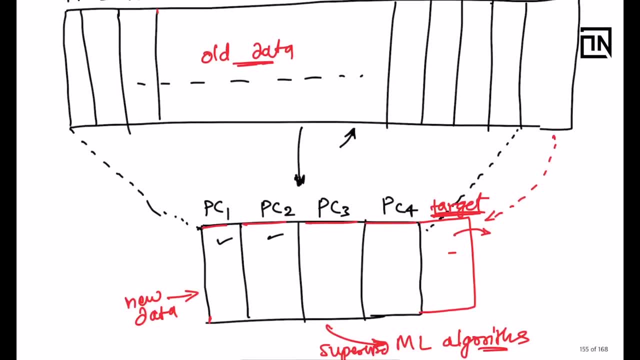 more columns. in order to find the best column out of it, or trying to find the equation of all the columns you will have, you will have to do more computations, and if you have less columns, then you will have to do lesser computations. okay, and your algorithm will. 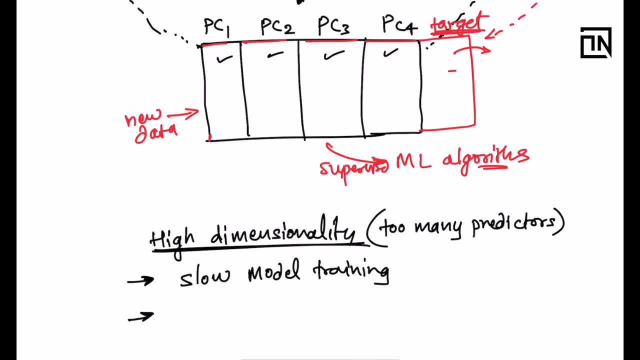 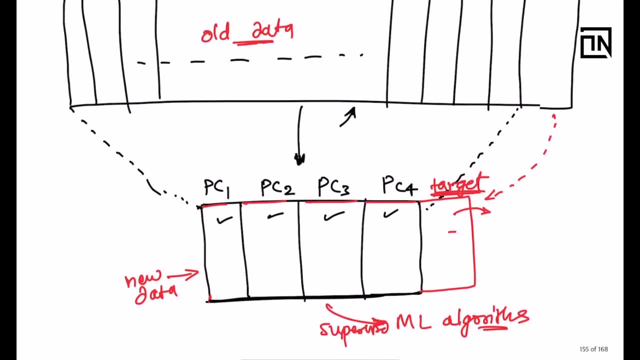 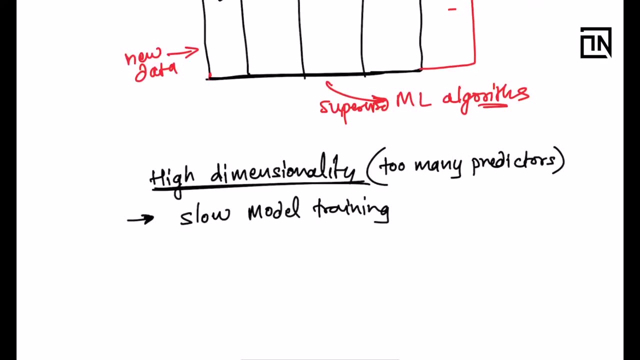 run fast. so once you convert your data into the reduced dimensions or a smaller version or or basically a compressed version of the overall data set, then you will be able to train your models very, very fast. and due to this slow model training, when your model is created, the model is also complex, which will also impact the time of predictions. so 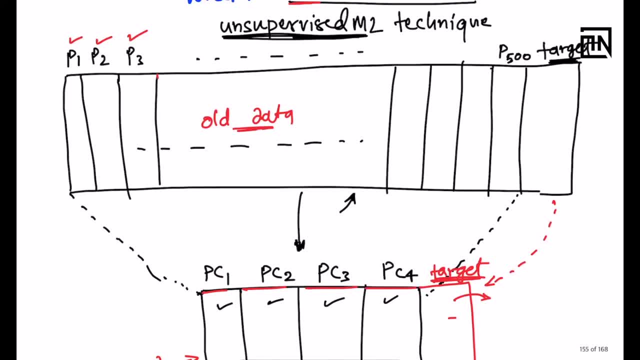 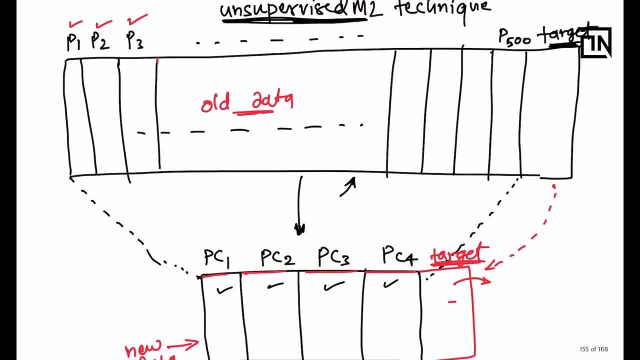 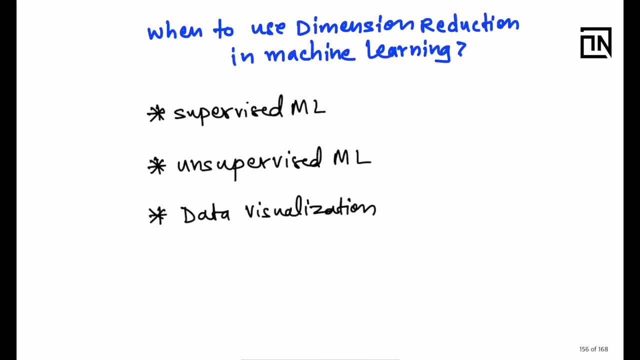 all these issues will come up if you have very high dimensionality in your data set and that can be resolved using dimension reduction, all right. so to perform this, there are many algorithms which are there, and i'll quickly describe them in the upcoming section. now let us discuss when do we use dimension reduction exactly? so we use it under supervised machine. 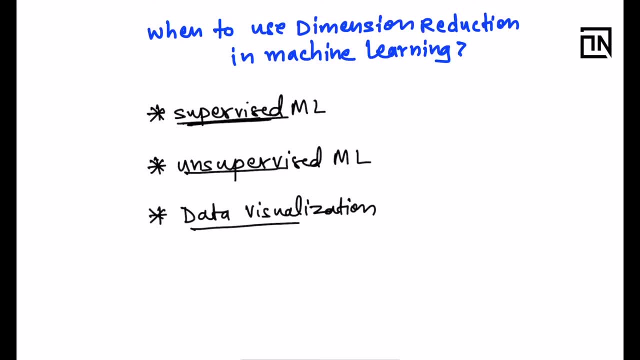 learning, under unsupervised machine learning and for data visualization. these are the three use cases where you can use dimension reduction, and every time the role of dimension reduction would be to reduce the number of columns so that i can do a better job, for example, in supervised machine learning. when exactly do you employ the dimension reduction technique? 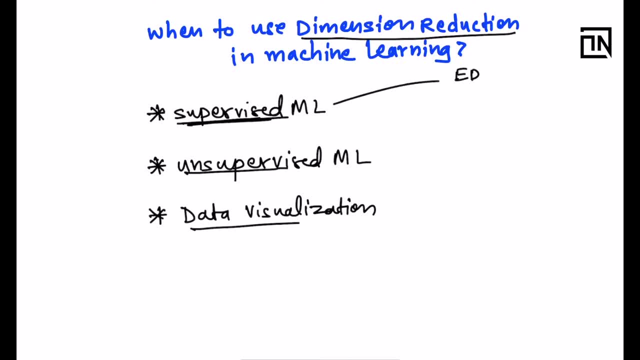 so in supervised machine learning, you have done your exploratory data analysis, you have done your correlation analysis, you have selected the feature and then you have converted the columns, the categorical columns or the string columns, into number. so often, what will happen there? there will be certain columns which have too many unique values, let's especially the string columns, and when you do get dummies, the number of variables will increase drastically after you do get dummies. so when each and every unique value becomes a predictor and then you have your target variable. so all obviously, it is high dimensional and the data has inflated. so in this scenario you can choose. 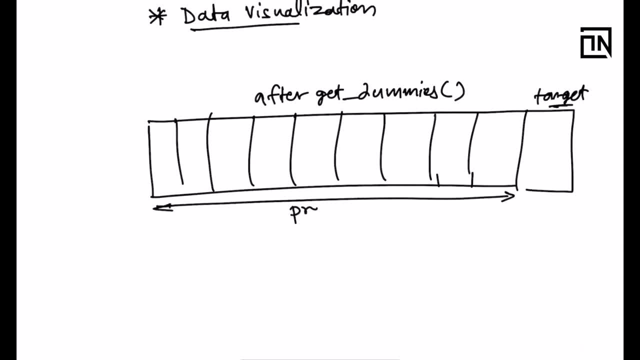 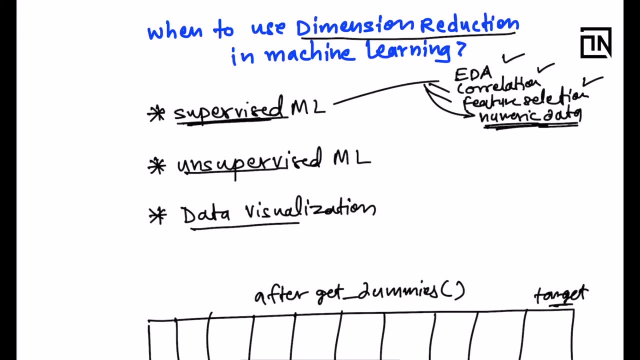 to shrink the predictors. so when do we perform this activity? only after all these things are done and you are at the verge of applying machine learning. so just before that, you take a call that there are too many predictors in the data. so let me try to represent them. 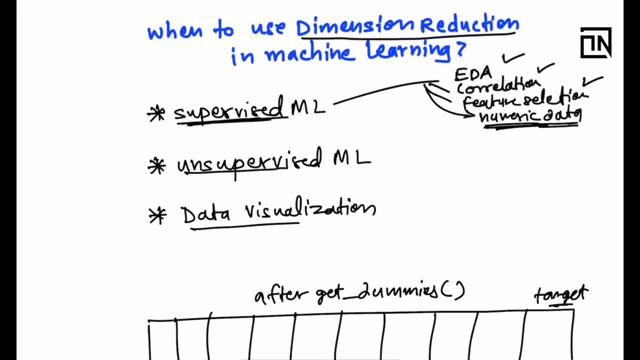 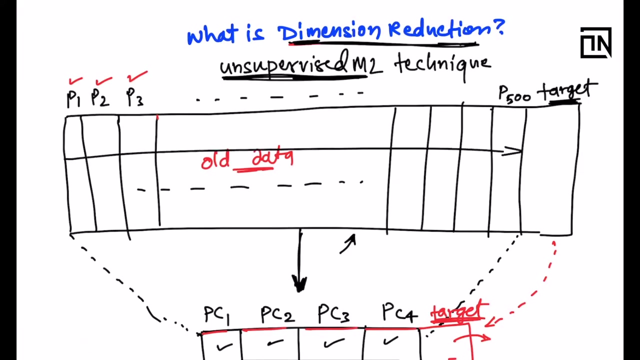 with smaller number of predictors. okay, you can take a call that there are too many columns. so instead of doing clustering on too many columns, let me shrink this data and do clustering on smaller set of columns. like, instead of doing clustering on all these variables, let me do the clustering only on these few variables. okay, I am just 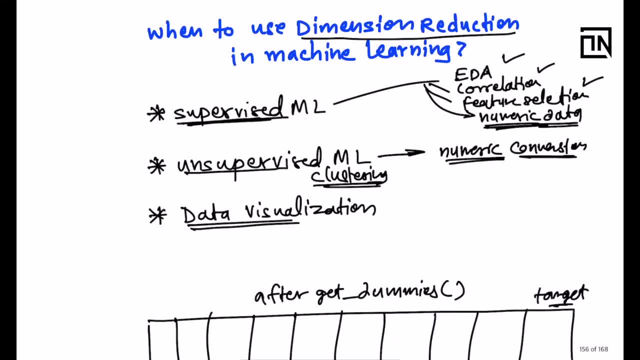 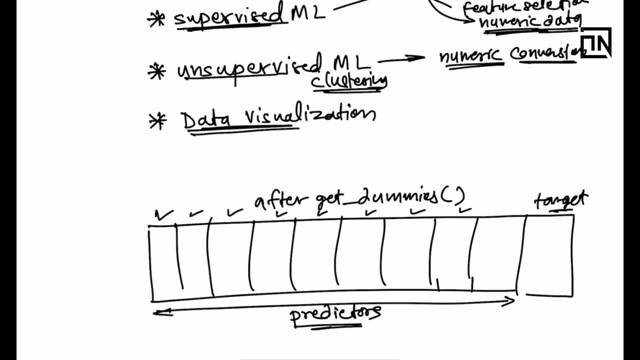 ruling out the target variable from the picture right now. similarly for data visualization. so if your data has too many columns, you cannot plot the n dimensional graph for all these columns, so it will be too computationally intensive as well as hectic to code. so if you still 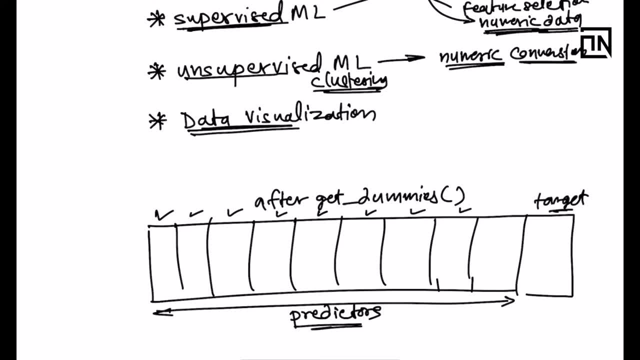 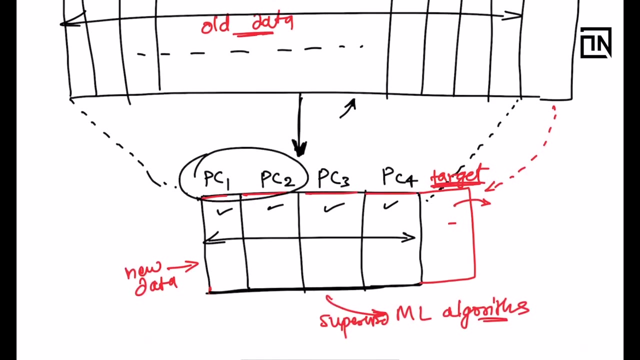 want to, if you still want to represent the data patterns or the data variations of all these columns using smaller set of variables. so all you have to do is just choose the first two principal components of first two factors which are really important. okay, so instead of using, let's say, 500 columns, all you have to do is just choose these two, predict these. 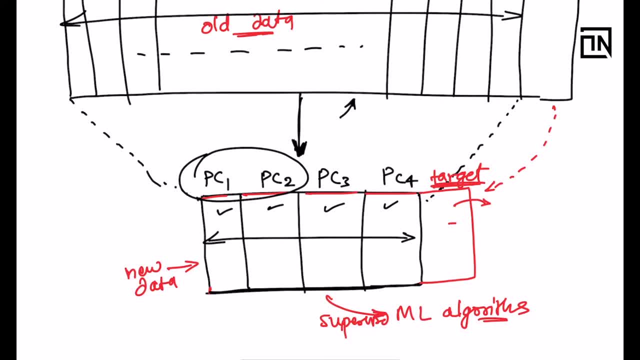 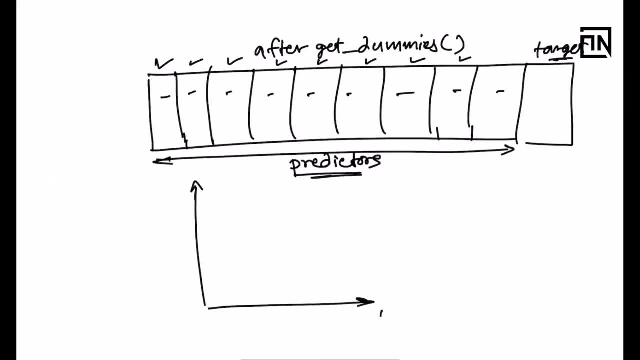 two factors which you have just generated, or these two principal components which you have generated, And then, based on this, you can create a chart which is two dimensional, so principal component one and principal component two, let's say, for example, so data can be visualized, its. 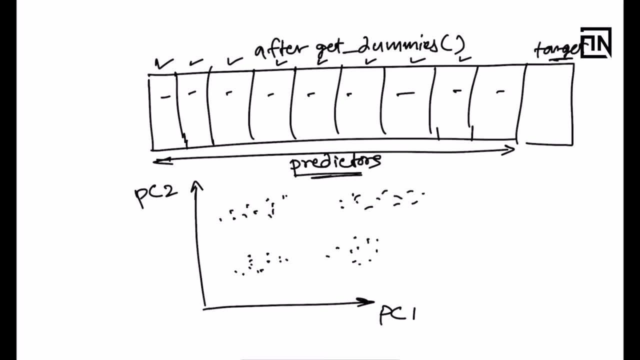 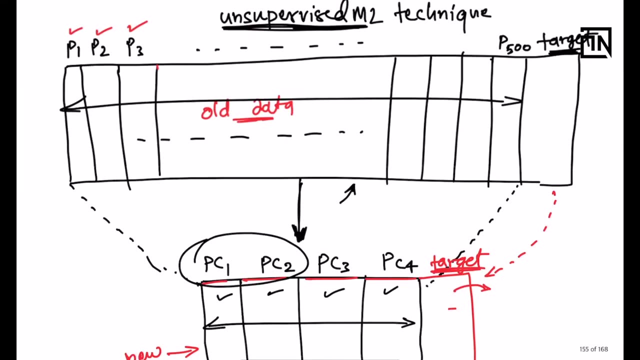 grouping can be studied and clustering can be observed. okay, so when you plot a multi dimensional data in lower dimensions, or just two dimensions, you don't just blindly choose any two columns. what you are doing is you are choosing a combination of such column because what pca? 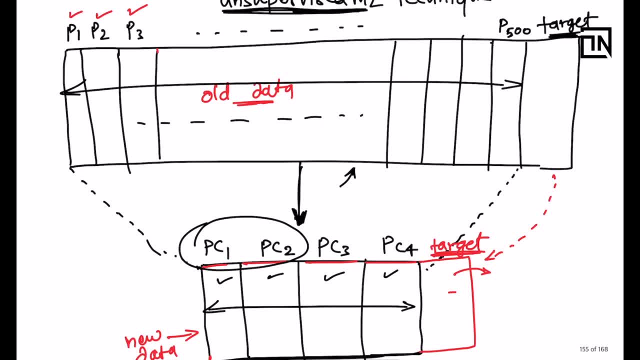 Or what factor analysis tries to do, is to represent multiple such columns as a single column. okay, so there might be redundant information in multiple columns which can be clubbed together and represented as one single principal component or one simple factor. okay, so combining multiple columns together, I will get my single column or single component or single factor. this. 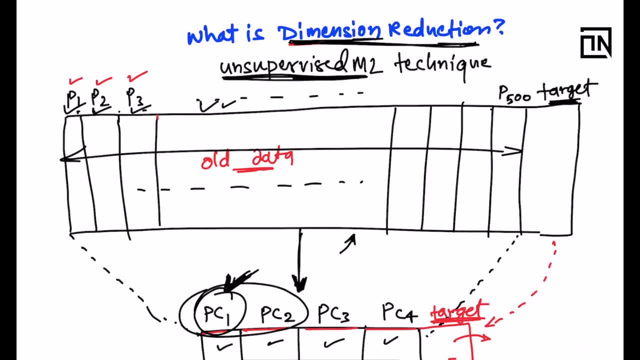 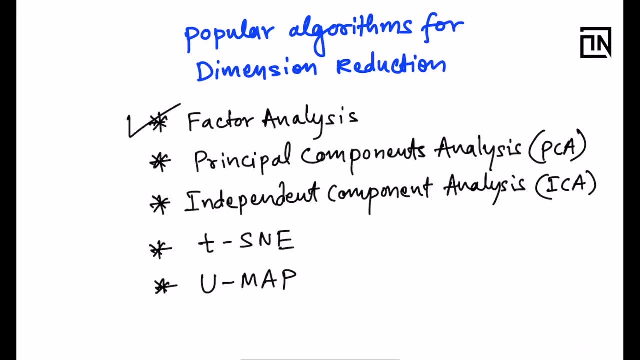 is what dimension reduction performs For you. okay, now to perform this, what are the algorithms do we have in place? so we have algorithms like factor analysis, principal component analysis, famously known as pca, independent component analysis, or ica, the t-sne, t-stochastic neighbor embedding, and last one is umap, which 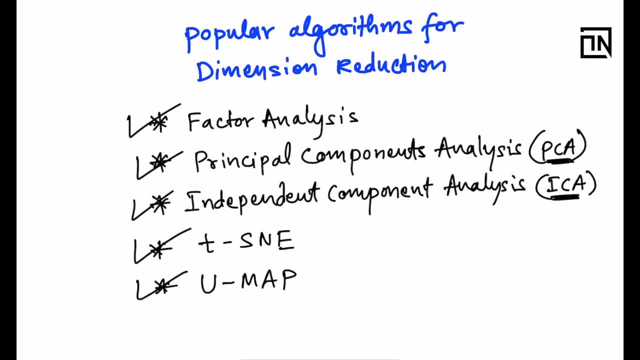 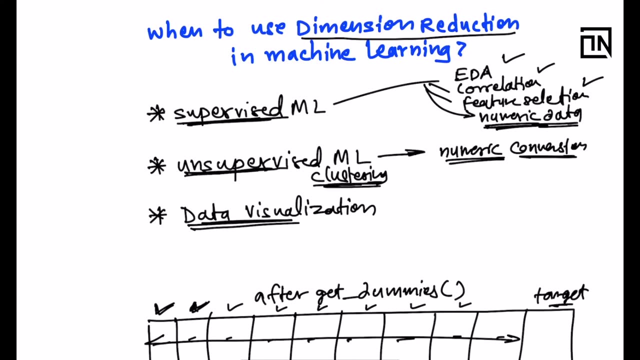 is uniform manifold, approximation and projection. So These two, primarily, are intended towards data visualization, But can also be used for supervised machine learning and unsupervised machine learning cases like clustering or let's say, in some kind of some form of natural language processing you are doing before doing classification or regression. okay, so in those scenarios also, 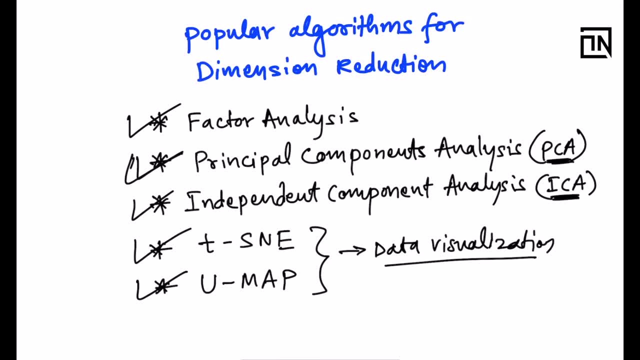 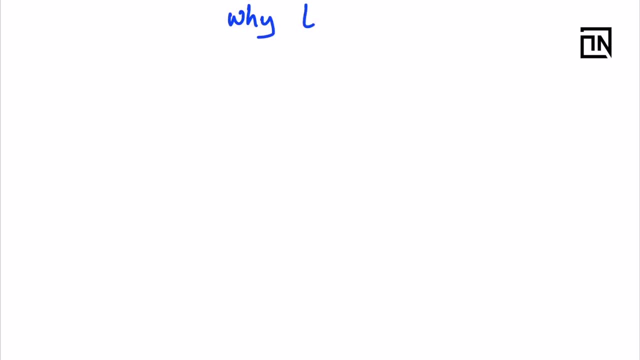 you can use this, but the most famous of them all is principal component analysis. So now let's try to understand. why do we need tsn? So This algorithm is focused primarily for visualization purposes, for data visualization. now consider this scenario where you have too many columns in the data. in your original data you have 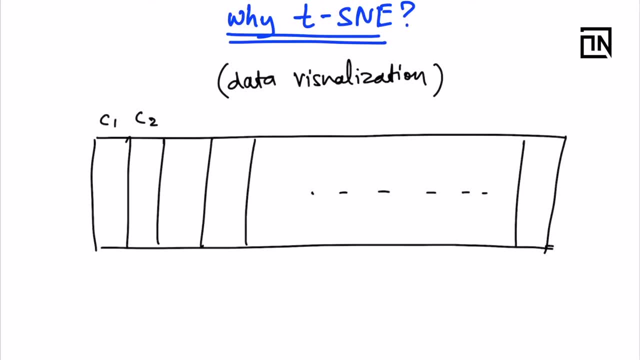 too many columns. let's say column 1, column 2, column 3, column 4: there are 500 columns. now, in order to visualize this data, all the all the columns put together, you will have to create a lot of charts. okay, to really understand how the crux of the data is, uh, or or to really 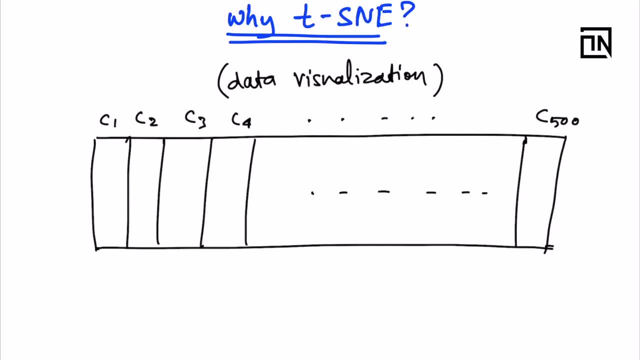 understand the data patterns present in this whole data. now sometimes, when we are trying to do clustering in those kind of applications, we would like to really understand how the data points are grouped together as a whole. so we would like to consider the variations of each and every column put together. now there are two choices: either we plot a five, 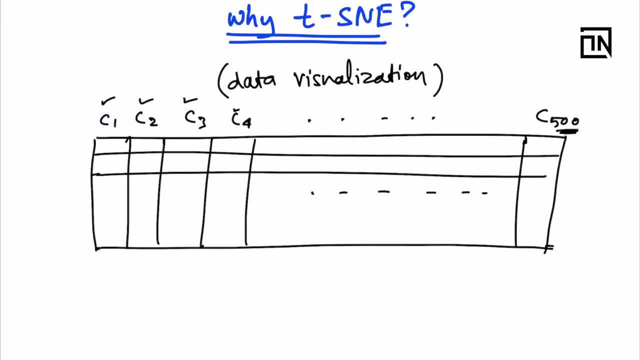 hundred dimensional curve which can give us an idea about how this data is grouped together, on which of which are the rows which are clustering together, which with each other, or we can choose any two columns, which is which is very common approach, which people take that choose any. 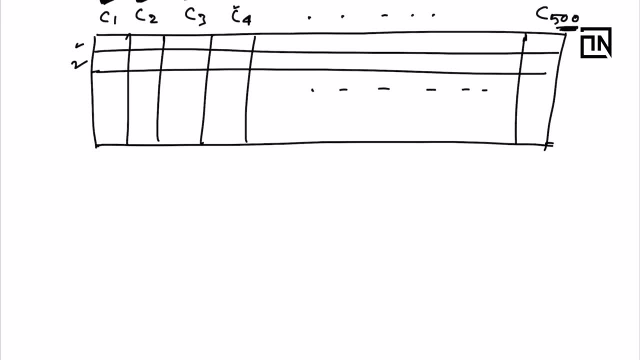 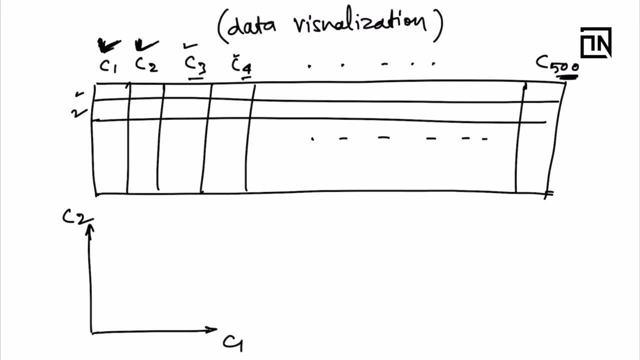 two important columns from this data and then just represent so. so what we'll try to do is we'll try to represent this data using, let's say, column 1 versus column 2, but we we know that this approach will lead to loss of Of all the other columns information and we will be representing the grouping information. 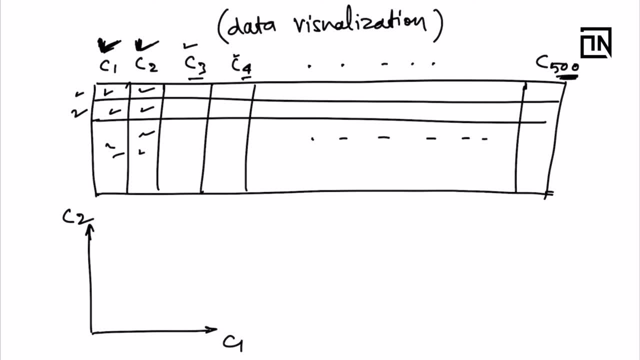 just based out of column 1 and column 2.. So is there a way wherein we can represent the information of all these 500 columns put together? So dimensional reduction comes into a picture. now, when we say dimension reduction, the famous pca comes to mind, so we can use principle component analysis to create a representation. 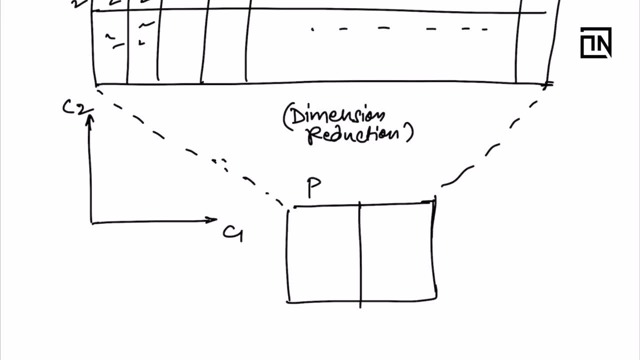 of this data contains lesser columns. let's say I created only two principal components and together they are explaining somewhere around 80% of the data variance and rest principal components I did not choose just for want of visualization. I wanted to plot principal component and principal. 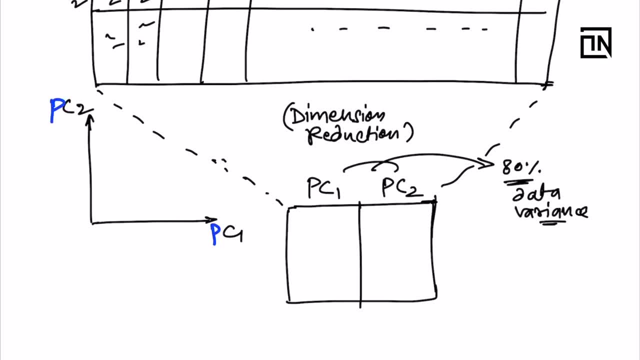 component 2, so principal component 1 and principal component 2 can be plotted and I will understand. okay, the data is grouped like this over here and it is grouped like this over here, like this group and one more group, so I will get an idea about the data as a whole, because 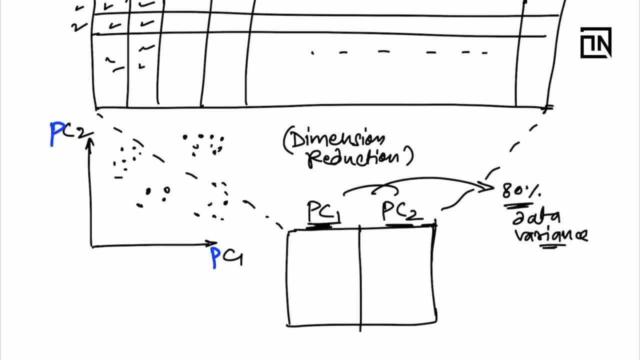 principal component 1 and 2. they collectively represent most of the data variance, so I get a good idea on how this data is clubbed or how this data is clustered or how this data is spreaded. basically, now, this can be done using PCA. definitely, but there is a limitation. 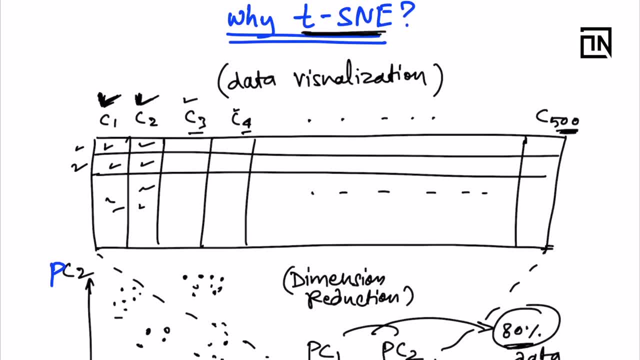 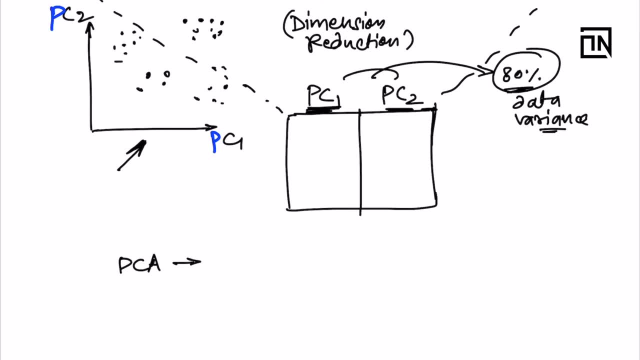 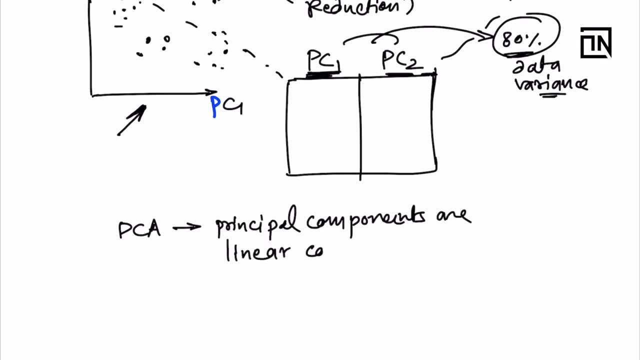 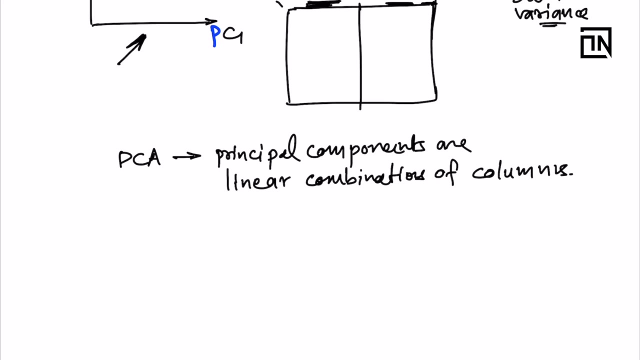 in PCA, which is improvised by TSNA. So PCA says. So PCA says PCA produces linear combination of the predictors or linear combination of the columns. so principal components are nothing but are linear combinations, whatever the columns you have in your data. but sometimes this may not be true. what if the data columns which we have has non-linear 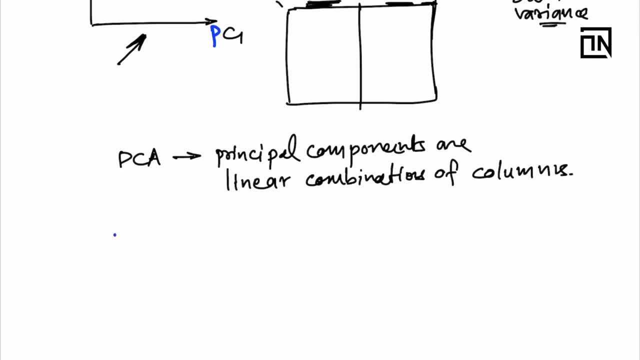 relationships between them. this is where TSNA comes into picture. this makes sure that whatever non-linear relationships are present in the data, they are captured. so we find components which represent or capture- you can say capture- non-linear relationships. so this is the main difference between TSNA and PCA and you can say this is one of the 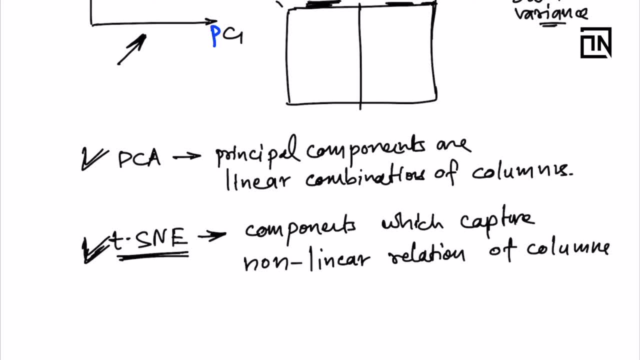 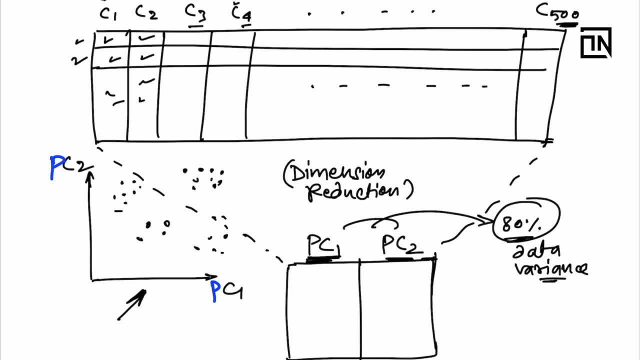 great advantages of TSNA that if it is able to capture the non-linear relationships of these columns, And we are creating two components out of it- let's say I created component and component two- and use those components to visualize my data in two dimensions, because typically 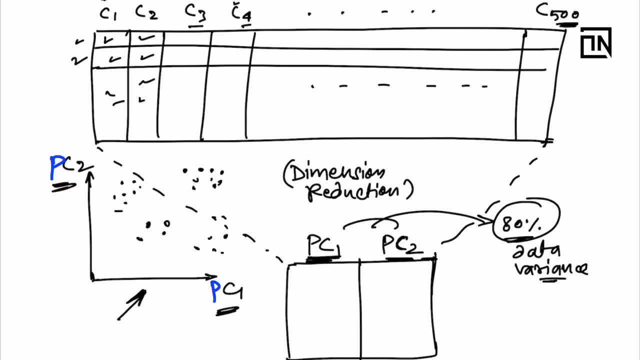 we will be concerned with two dimensions. we will be plotting two dimensions mostly because it's easy to plot. we can do one more dimension, we can plot three columns or three principal components or three components of SNE, But then that will also be a little extra work. so people usually stick to two dimensions. 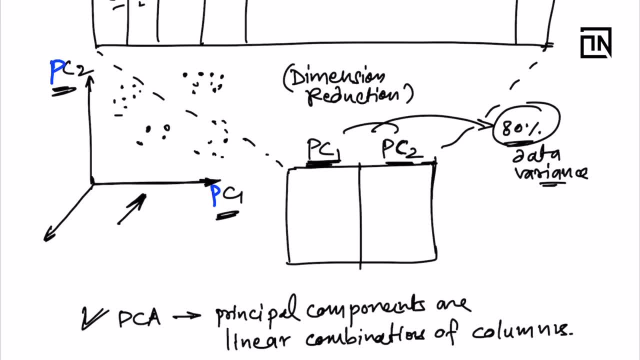 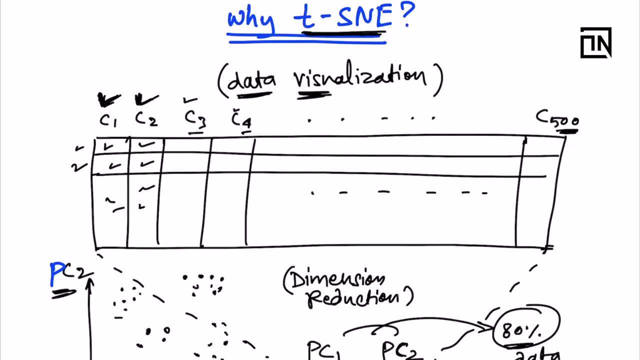 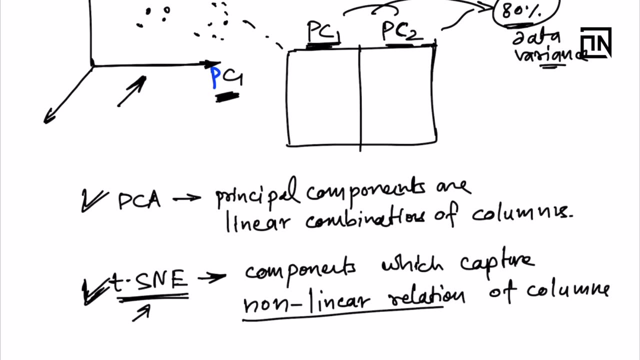 it's easy to visualize And To explain to someone. So maximum two dimensions are what we target whenever we are trying to visualize any given data, especially when we are trying to understand how the grouping is. So this is where TSNA is really helpful, and I gave you the crux already that it captures. 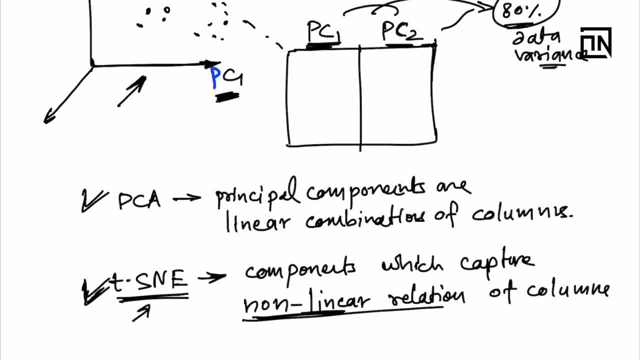 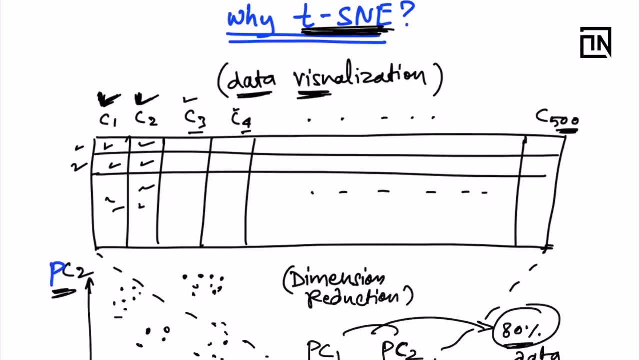 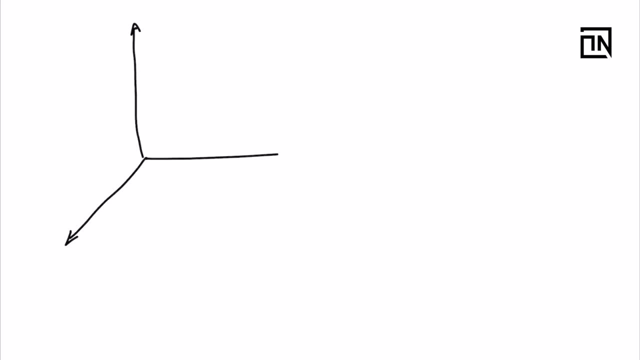 the non-linear relationship of columns. So now let's understand how this exactly works. what are the steps, what are the methodologies which are behind this algorithm? So consider a very simple scenario. There is a data set which contains three columns, so you can plot it in 3D. 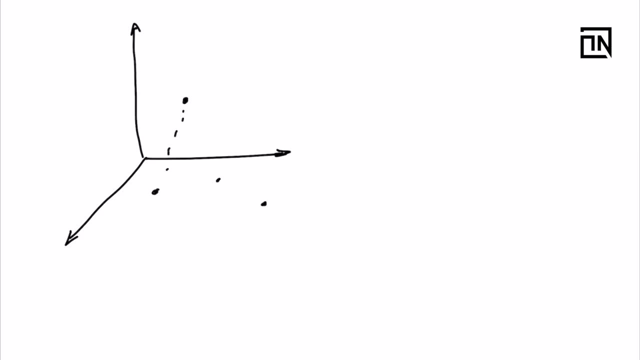 So one point is here. one point is here. one point is here: you can plot this data into three dimensions. Okay, now you want to represent this data in just two dimensions. instead of three dimensions, you want to represent it in just two dimensions. So, as I described, one way is to just select two columns out of the data or try to find. 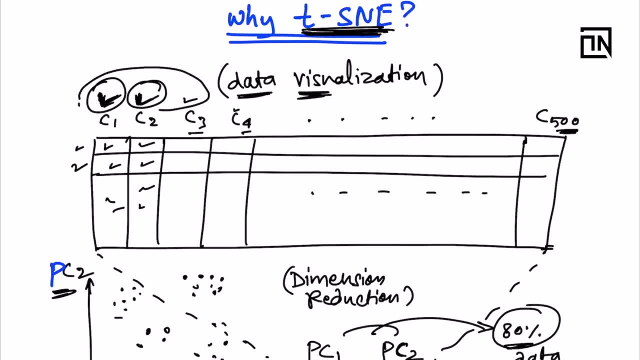 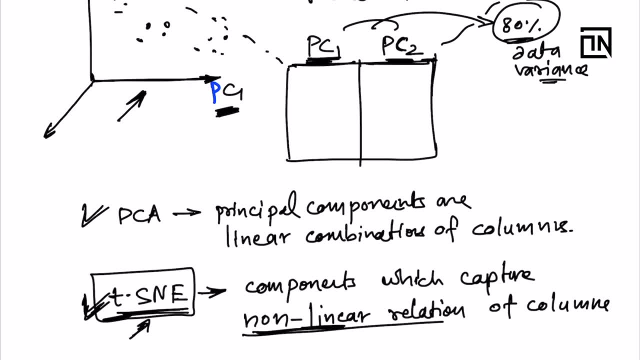 a representation, One of these three columns put together as two columns, like two components. So you can do it with PCA as well as you can do it with TSNA. So if you do it with TSNA, what will happen is it will maintain the kind of relationship. 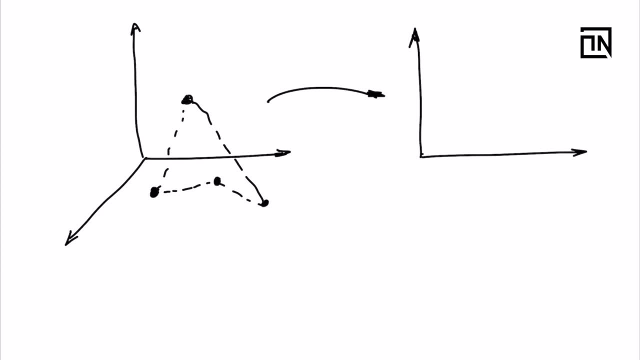 these points had in three dimensions, in two dimensions as well. I repeat, TSNA will conserve the kind of the kind of relationship or the kind of you know you can say, distribution we had in three dimensions or n dimensions, in multiple dimensions. it will retain that in two dimensions also. 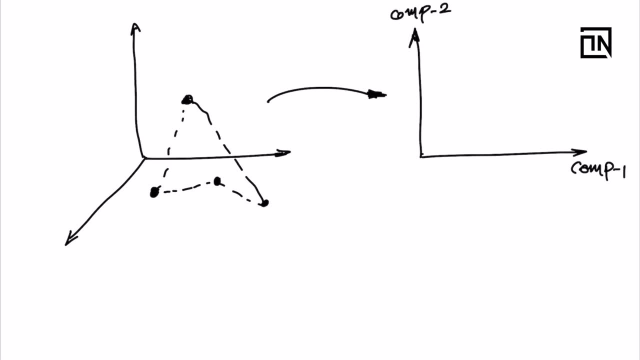 So the component one and the component two, which we will create it, will have a similar kind of distribution in two dimensions for this data, So the topology might be little different, but the overall properties will be same of the data, So the representation will be more accurate. 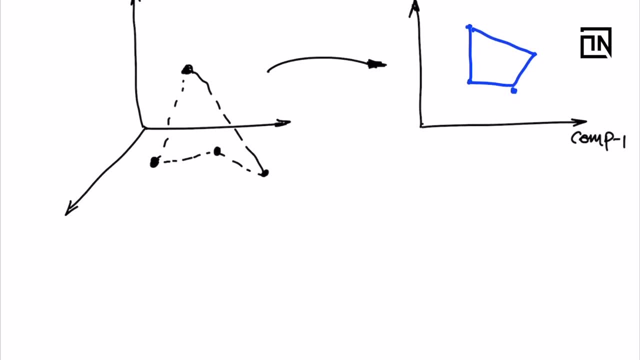 Now how this is achieved is In three dimensions. Let's say I have the Euclidean distances from point, let's say point number one, two, three, four. So I'll compute the Euclidean distances for each point: from point one to two. distance between point one to two. distance between point two to three. distance between three. 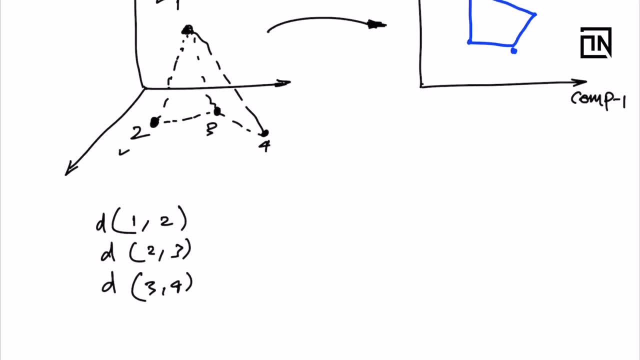 to four, even one to three, one to four, so on and so forth. So every pair which you can find, You will compute the Euclidean distance. So you find this Euclidean distance and based on this distance, you can find the probabilities. What are these probabilities? probabilities of these two points being close. 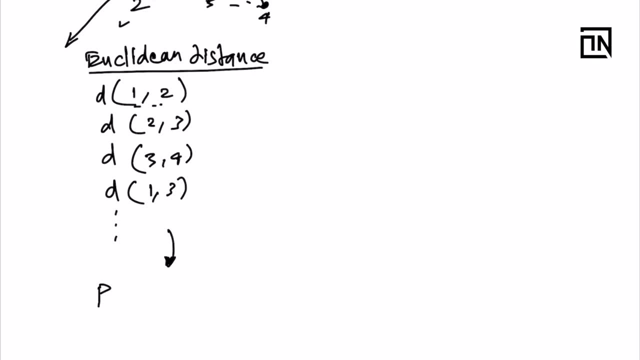 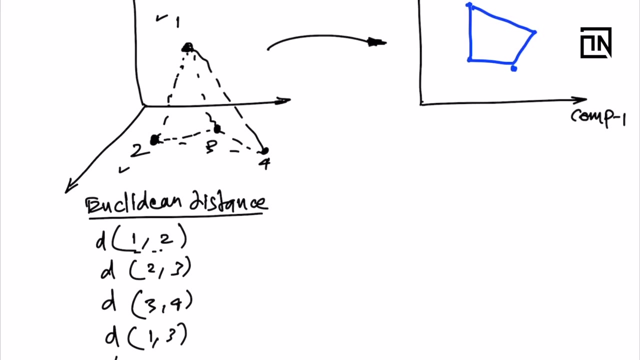 So you can measure the distance versus all the other distances and you can calculate a probability of one and two being close, a probability of two and three being close, so on and so forth. So this is being done in the high dimension, or you can say three dimensions right now. 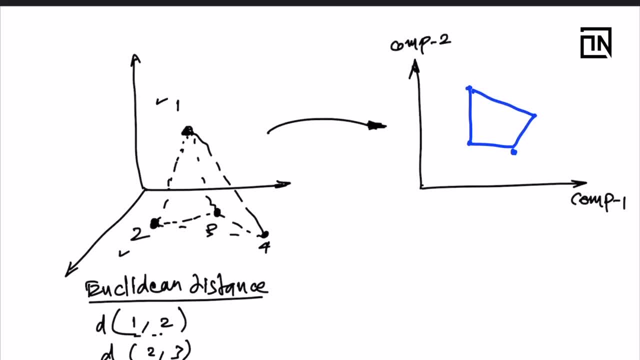 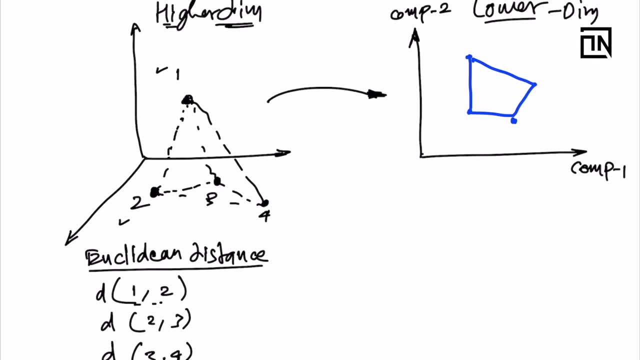 and the same activity is done in lower dimensions also. So this is my lower dimension and this is higher dimension. So here I am having only three columns and I'm trying to represent it with two columns, and this scenario could be more complex, like my higher dimension has 10 columns or 200. 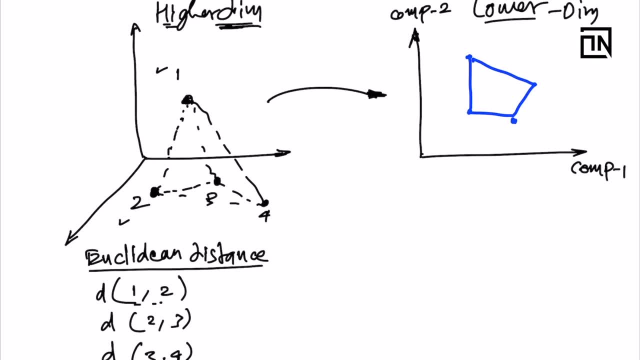 columns, or 500 columns, and I'm trying to shrink it down to two columns, Only two components. So in that scenario also, I'll be representing my whole data with just two components. and why this is why this is only two, why it can't be three, it can be three, it can be four also. 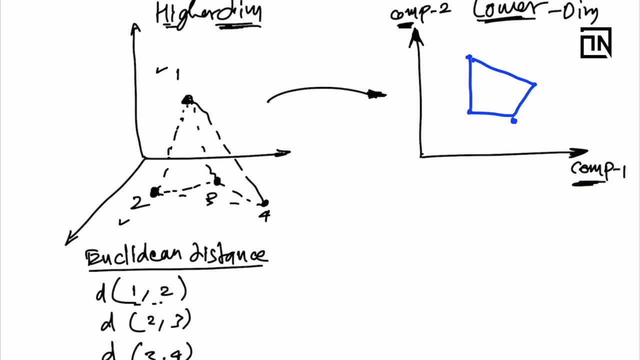 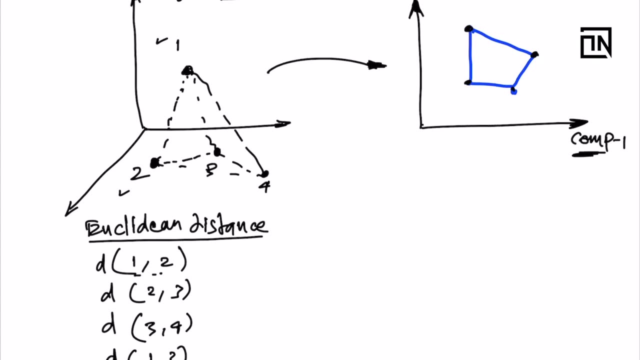 but since I'm targeting to visualize the data, two components make more sense, So I'll always try to represent my data with two columns. So once you do this, the topology of the data is created in such a way that the Euclidean distances are scaled. 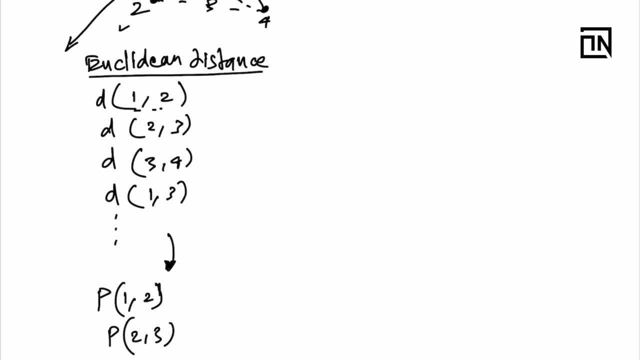 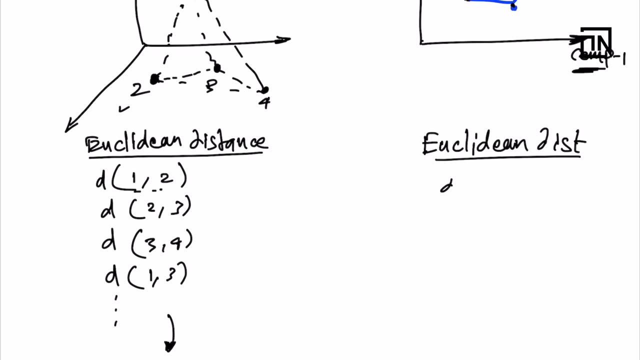 In a way that probability, which you got in higher dimension, is present exactly in the same fashion in the lower dimensions also. So what is the driving factor of T-SNE algorithm is it also calculates the Euclidean distance over here. So distance of, let me call this point one, two, three, four. once again, distance of one. 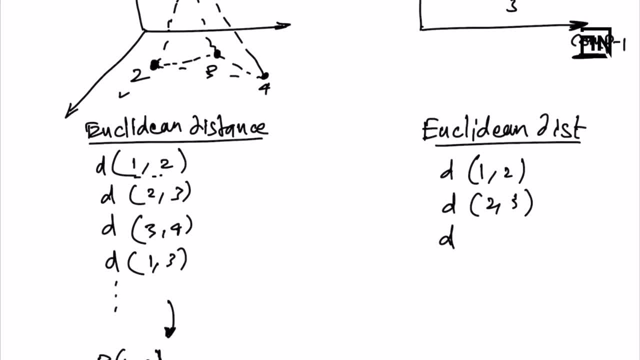 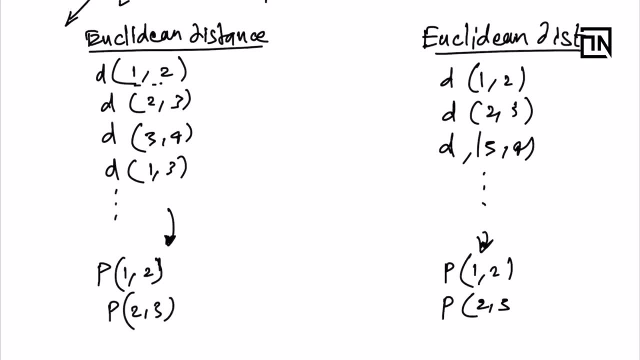 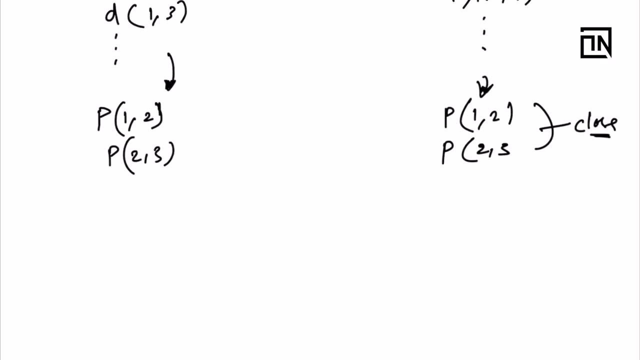 to two, distance of two to three, distance of three to four, so on, so forth. And then it also calculates the probability being close together. And now it shifts these distances in the lower dimension in such a way that these probability, like if this probability was zero point eight, or zero point three, then here also it should. 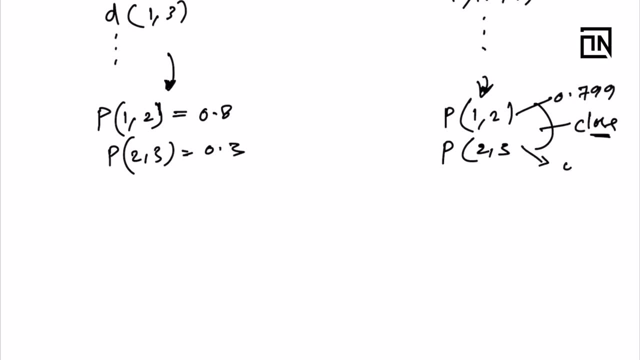 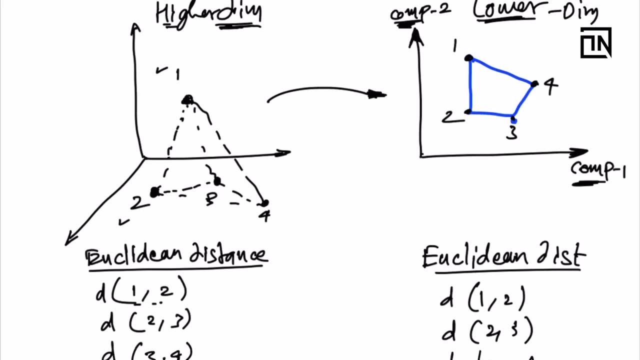 come close to, let's say, zero point seven, nine nine, or zero point two, nine, nine. so very close. It should come close to the probabilities in the higher dimension. Once this is done, the topology will represent The exact, Similar kind of properties which you had in higher dimension scaled down to lower dimension.